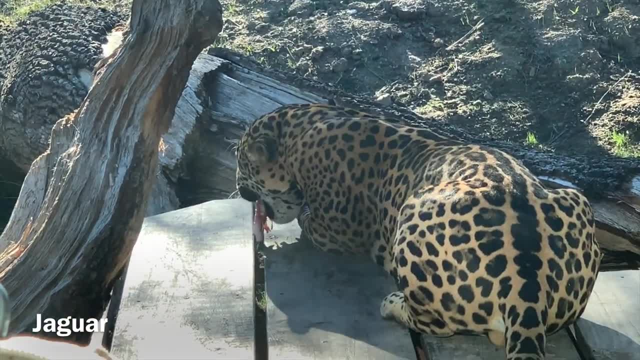 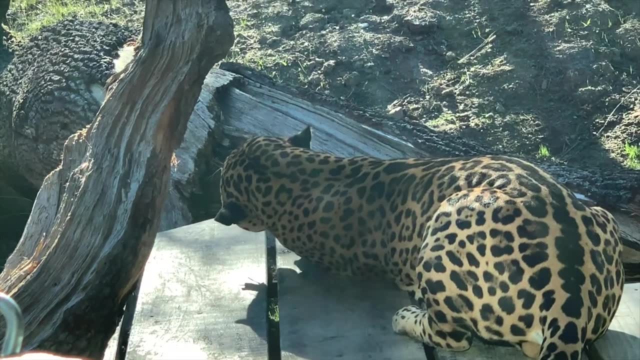 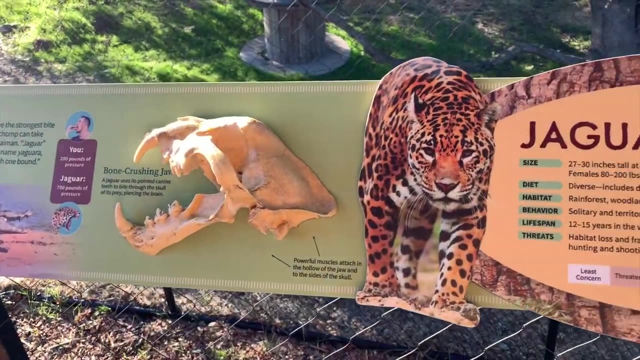 Next we spot the jaguar. Yes, this animal once lived in California. In fact, in the early 20th century the jaguars range extended as far west as Monterey in Northern California. They're now endangered due to hunting. Jaguars used to be native to this area. 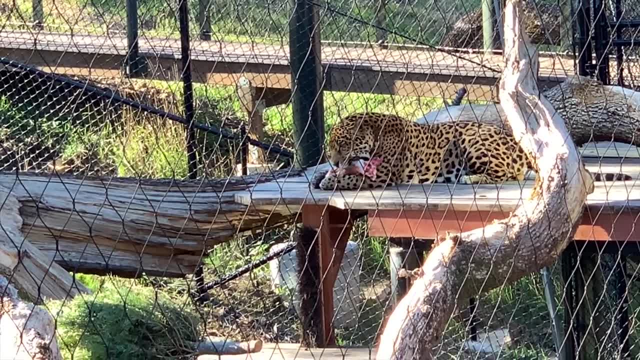 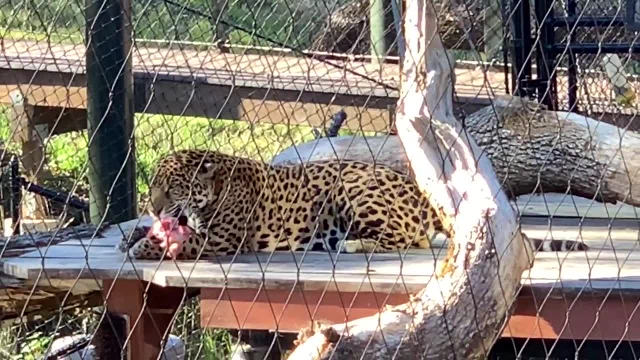 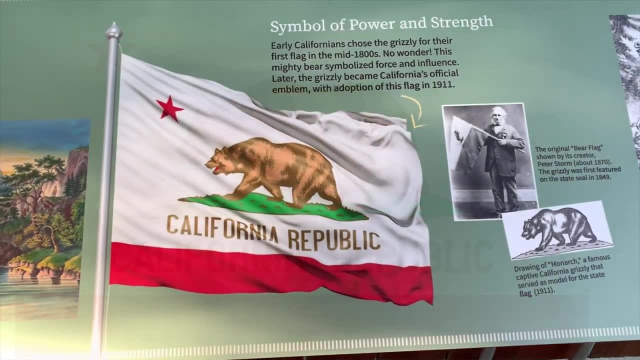 Historically, wildlife conservationists are hoping that this exhibit will raise awareness so that these animals can thrive once again. Now for one of California's most visible and enduring symbols, the grizzly bear. But where have they all gone Prior to the Spanish settlement in? 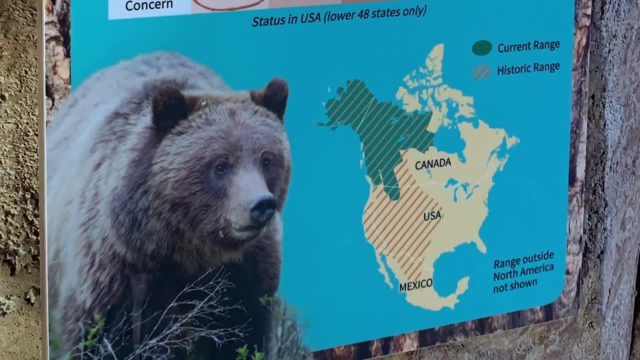 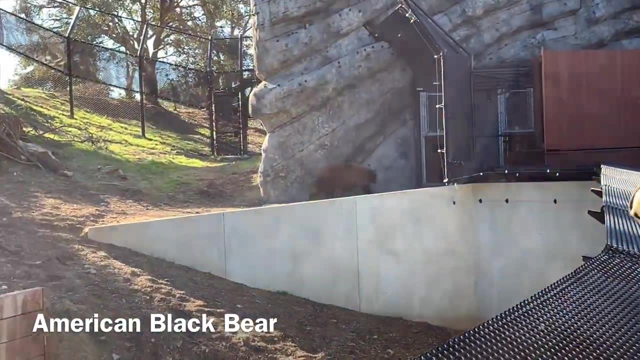 the 18th century. there were roughly 10,000 grizzlies in California less than 75 years after the discovery of gold in 1850.. In 1848, almost every grizzly in California had been tracked down and killed After the 1920s. 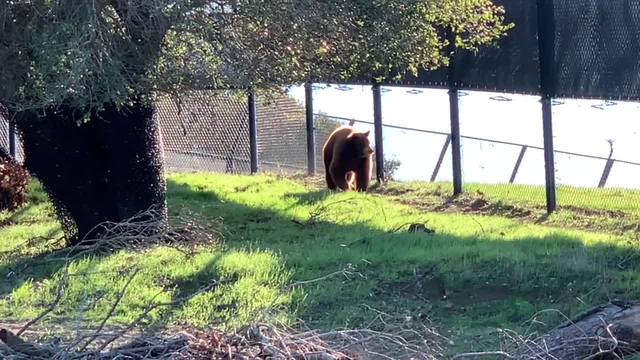 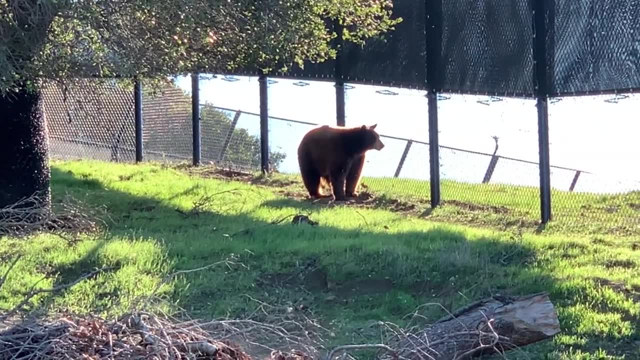 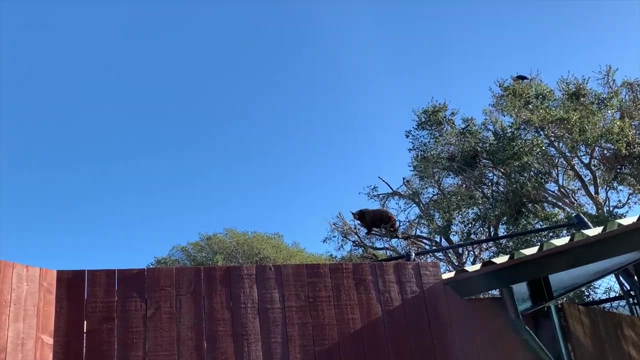 no grizzlies were ever seen again Prior to visiting the zoo. I never realized that the grizzly which is seen on our flag in numerous California sports teams cannot even be found in our state. The zoo rescued this black bear after it was threatened for being euthanized. 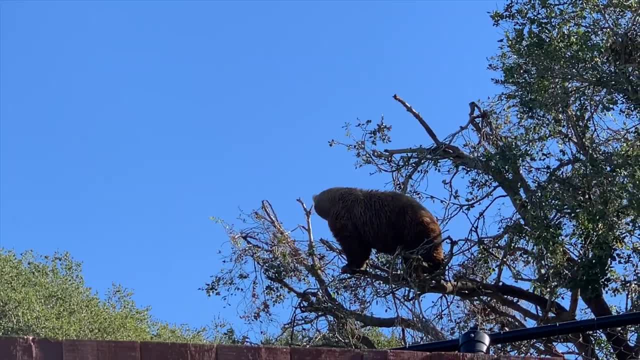 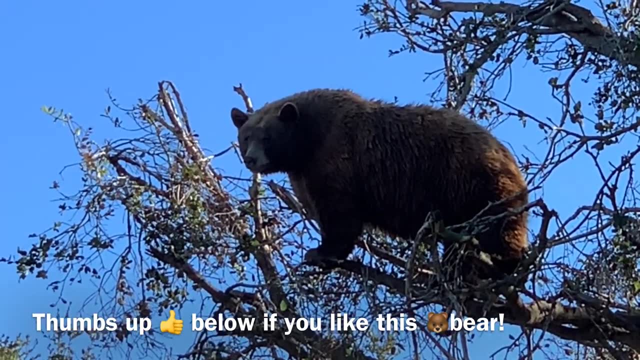 after invading on a black bear, The grizzly bear was found in California's California National Forest Service. The grizzly bear is now a home. Now the bear is safe here and climbing trees. I've visited many zoos before, but this was my first time seeing a bear in action climbing. 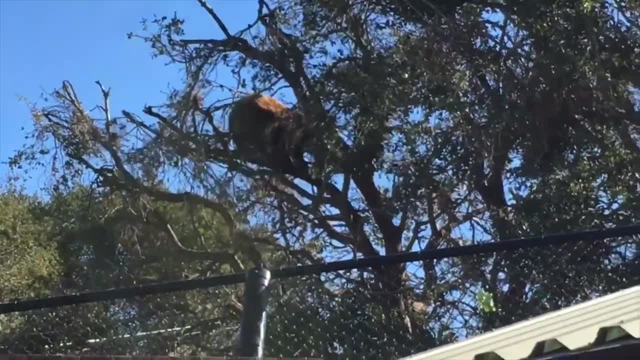 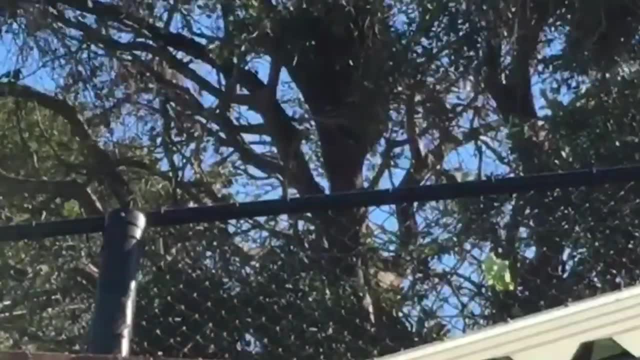 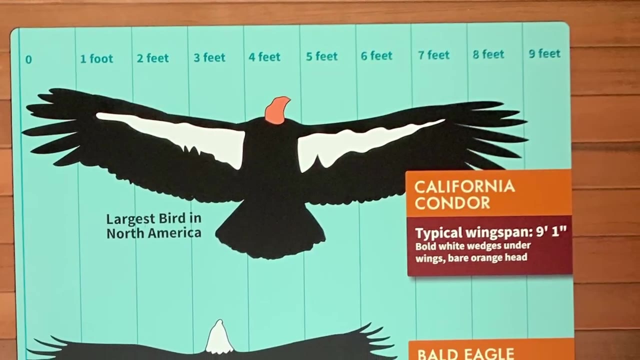 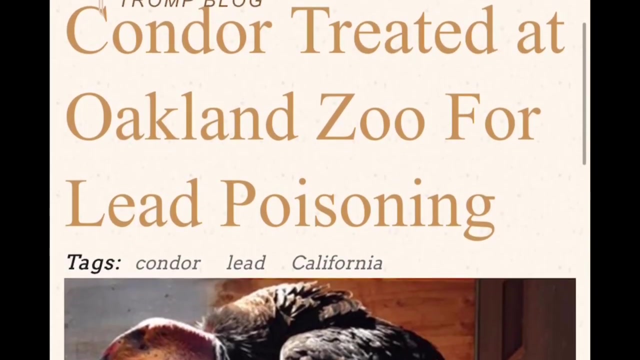 a tree. The zoo hopes that you can see these animals for yourself, make a connection and help protect them for the future. One of the greatest success stories of the zoo is the story of the California condor. In 1987, they were almost extinct, with only 27 left in the wild. They were brought to 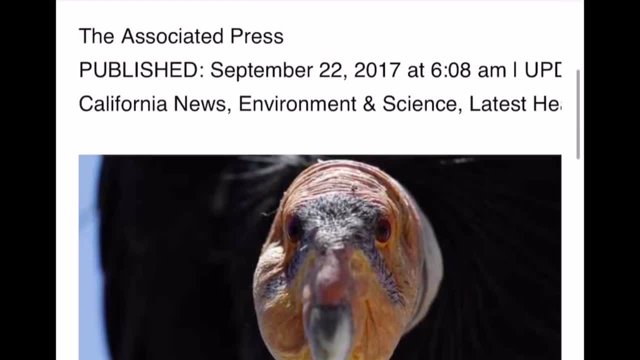 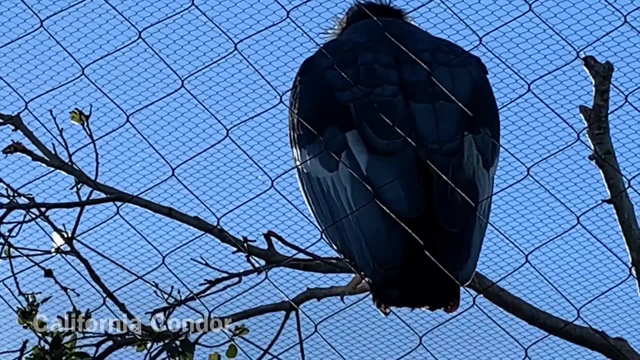 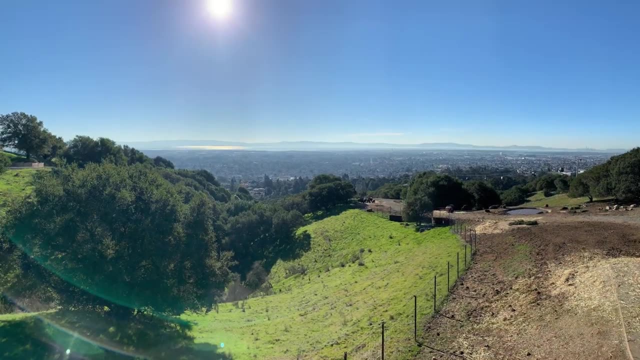 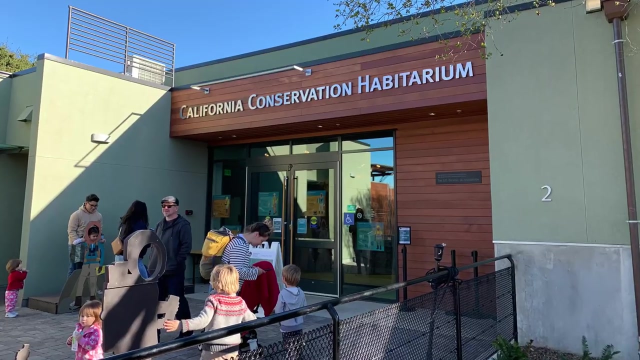 the zoo, treated for lead poisoning and now making a comeback. Gosh, look at that. His head turns all the way around. Now for one of the most breathtaking highlights of the zoo: the panoramic view of the Bay Area. Welcome to Tools and Dreams. 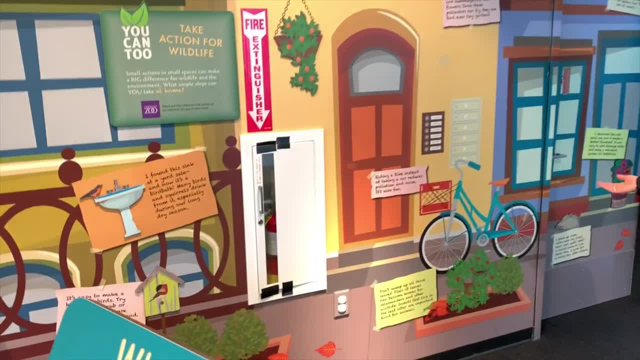 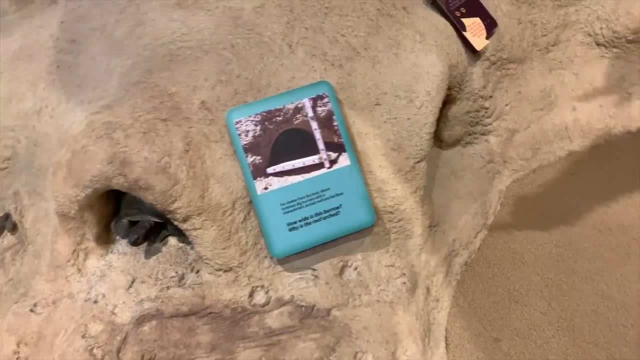 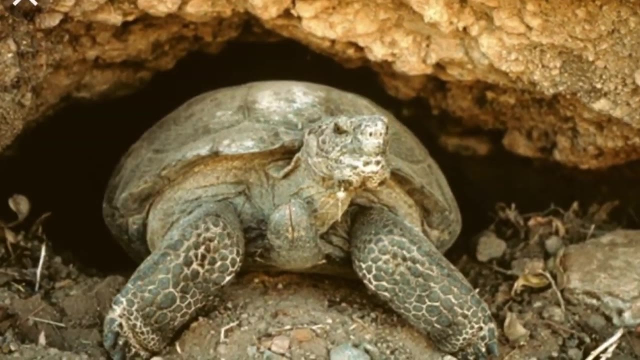 The zoo also teaches the next generation what it's like to be a biologist through a very interactive exhibition called The Habitarium. The exhibit teaches kids how to explore nature and respect the environment, And we talkt about what the biologists are looking for in that burrow and that shape. 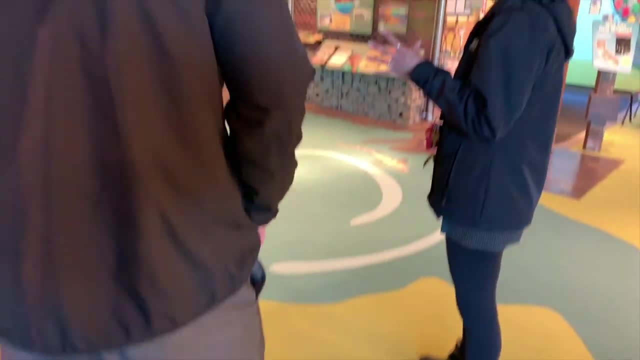 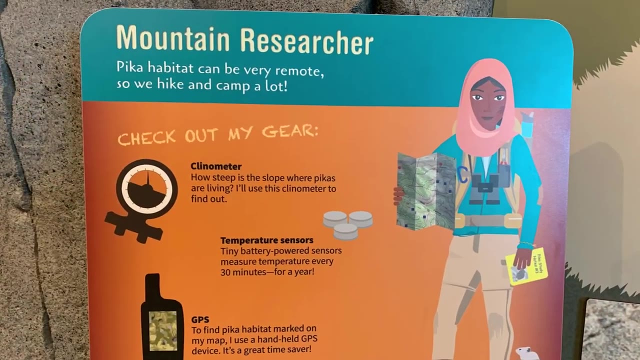 when they're out there, because they spend most of their life underriz, Mmmm, Mmmmmm how connected we are to our environment and gives them ideas on how we can take action and also sparks an interest in stem careers such as biology. 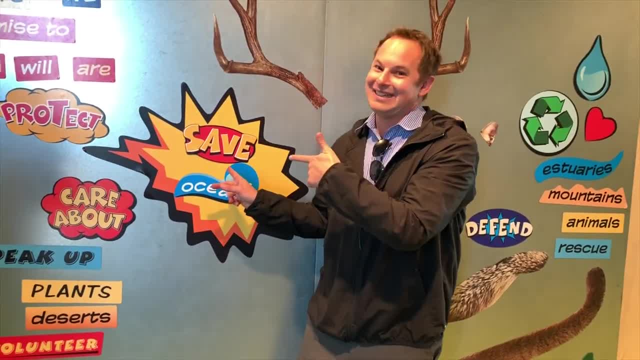 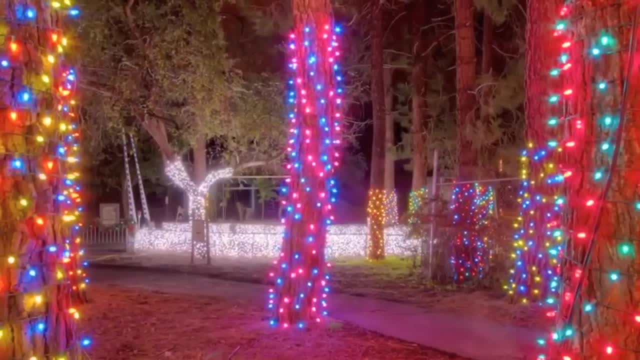 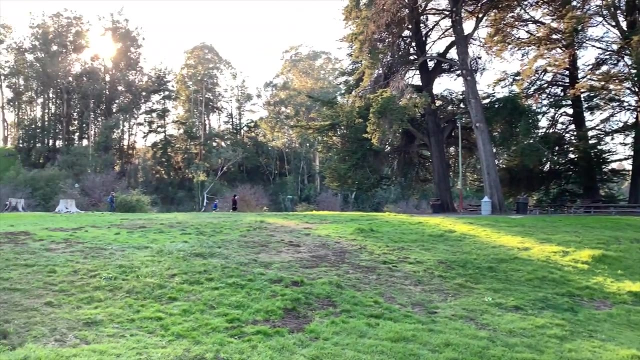 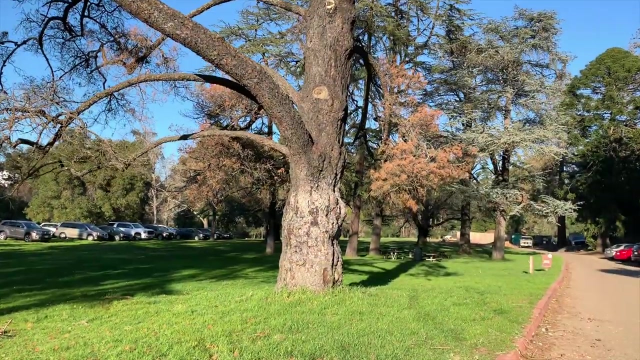 you're an action hero, i'm committed. and during winter time they have the oakland zoo lights at night. the oakland zoo is perched high above the oakland hills and you can bring some food here and have a picnic. and there's also lots of trails, too, surrounding the zoo. did somebody say trails? 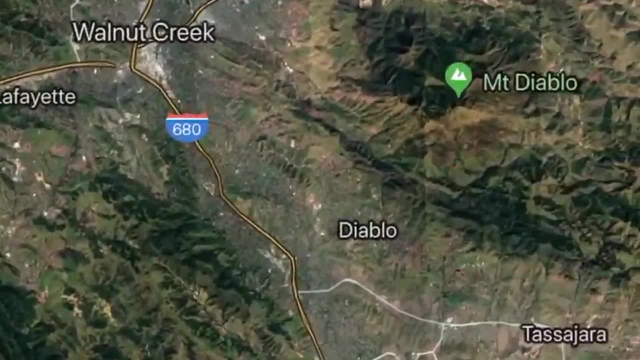 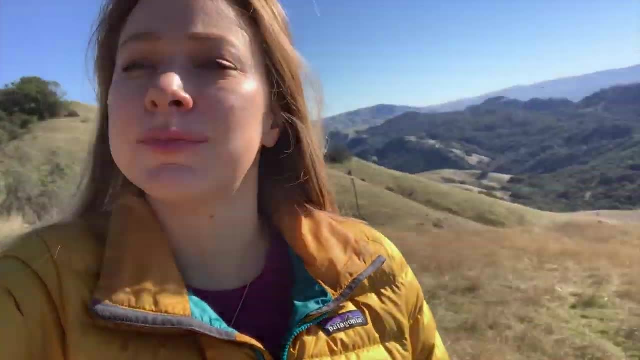 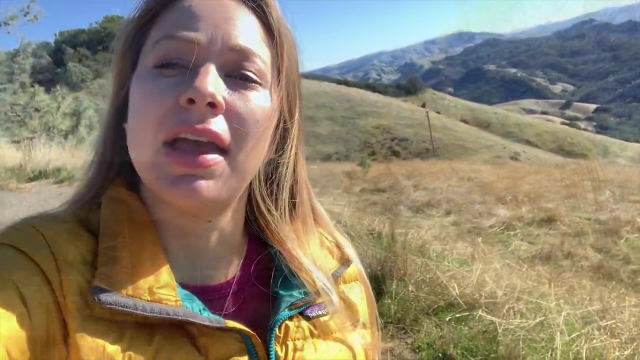 it's time to head one hour inland from the oakland zoo to mount diablo, one of the highest peaks just drove up to a place in the east bay called mount diablo. it's really high up, over a thousand feet, and the view is of the entire east bay. 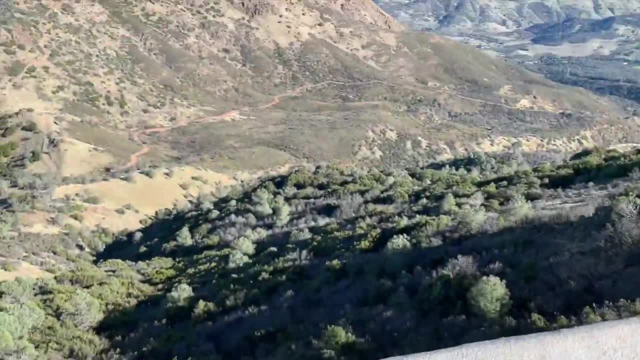 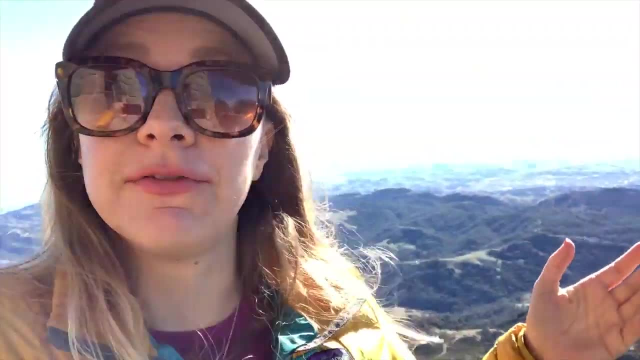 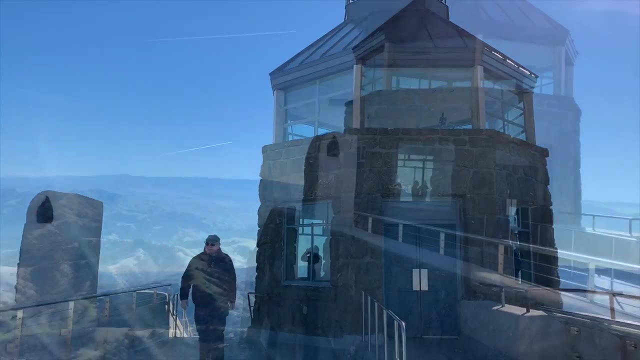 look at how green the hills are. this is late december here. this is the summit of mount diablo, 3849 feet high. this is the trail a lot of people like. up here there's a lighthouse. we're at the top of mount diablo and behind us you can see. 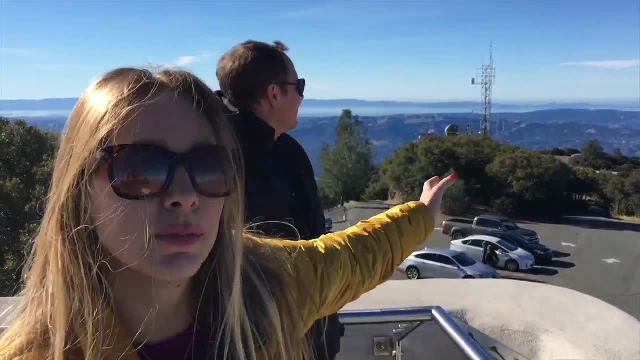 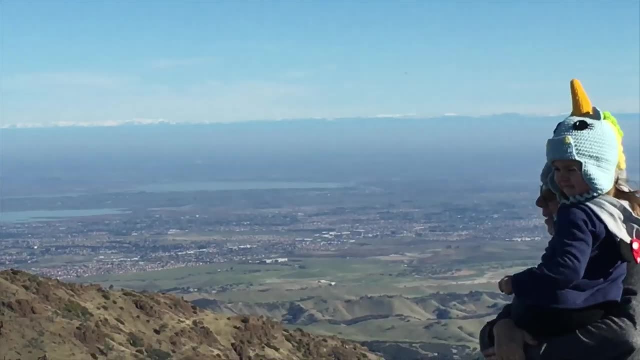 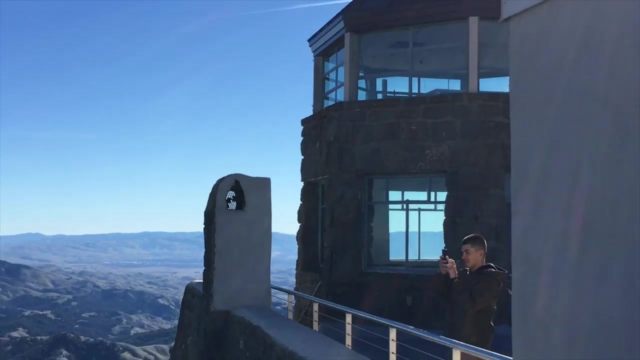 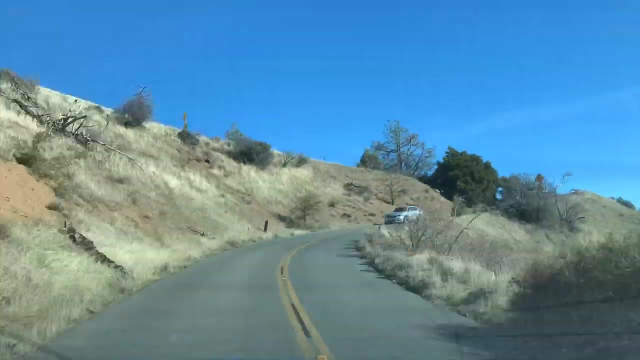 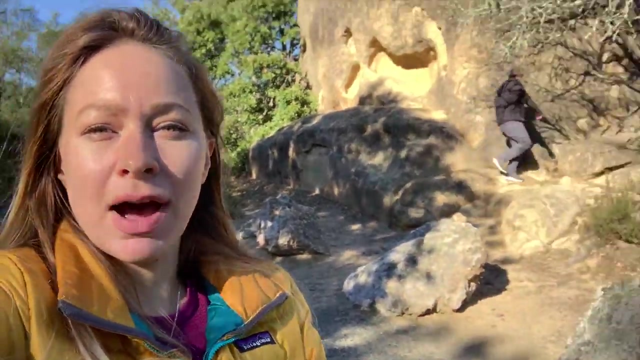 the city of san francisco. look at how small it is from up here. if you like these views as much as we do, be sure to hit the thumbs up button down below so you can see. it's not too far off, but it's not that far away.